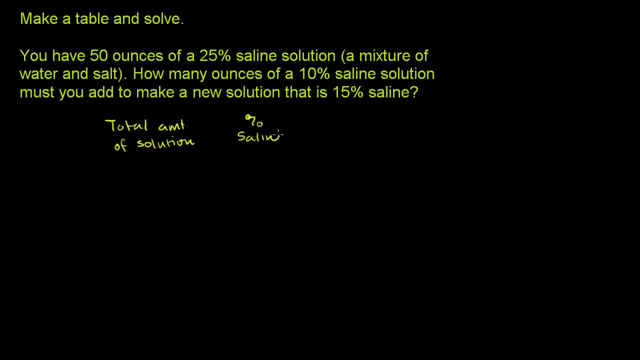 So percent saline, And then we can use this information to figure out total amount of saline And let's list it for each of the two solutions that they talk about. We're starting with 50 ounces of a 25% saline solution. So this is what we start with. 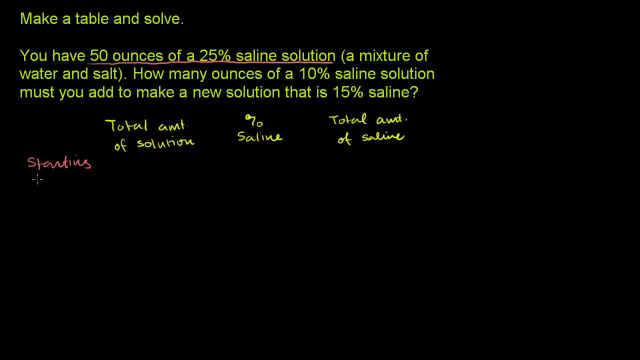 We start with this starting solution. We have 50 ounces of it, So I'll just write 50.. We'll assume everything is in ounces. It is 25% saline. So if we wanted to figure out the total ounces of saline, we 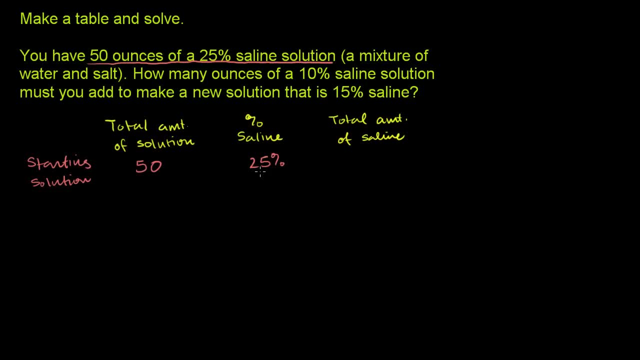 say: well, we have 50 ounces. Multiply that by 25. And we have the total amount of saline in this solution. So 50 times 25%, that's the same thing as 50 divided by 4. So that's 12.5.. 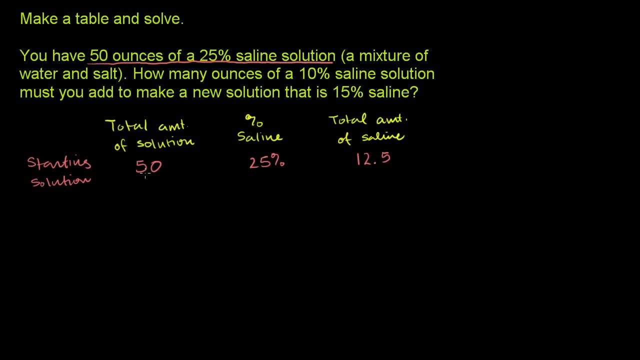 So that's 12.5 ounces of saline in this 50 total ounces, It's 25% saline. Now let's talk about what we're going to add to it. We are going to add, so solution added. Now they say how many ounces of a 10% solution? 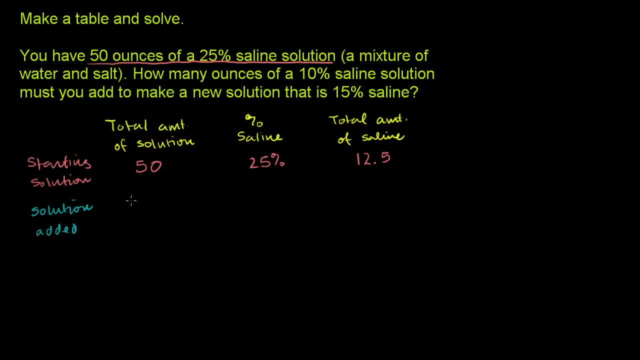 So we don't even know how many ounces we're going to add. That's what we have to actually solve for. So let's call that x for the amount of solution that we have to add. So we don't know how much we're going to add. 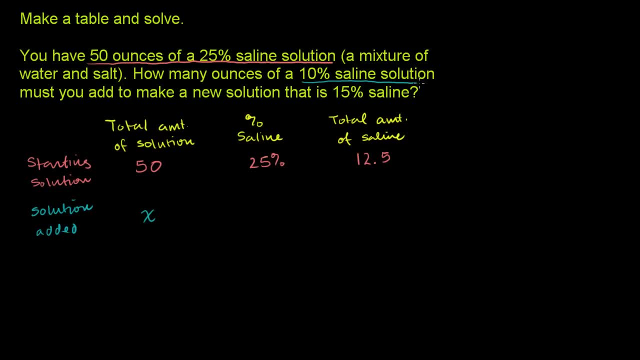 But we do know that it is a 10% saline solution. We do know that it is a 10% saline solution And if we know what x is, we know the total amount of saline is going to be the 10% of x. 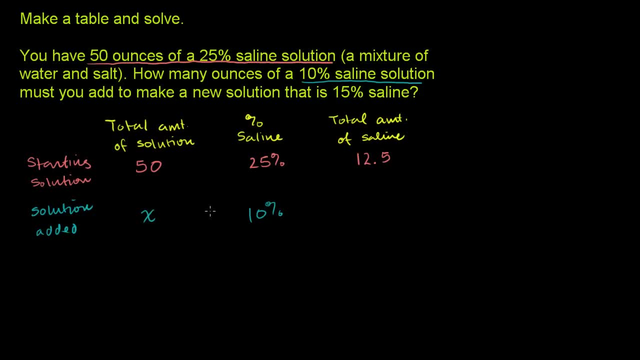 If we have- I don't know what this is- If we had 50. We have 50. If we had 50 here, it would be 10% of 50. If we had 10 here, it would be 10% of 10.. 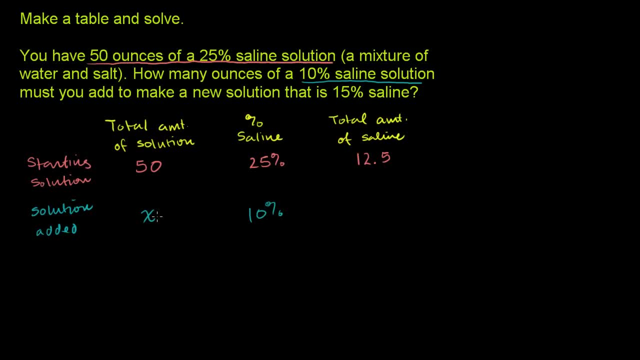 So the amount of saline we have in this solution in x ounces of the solution is going to be 0.1x or 10% of x. That's what 10% of the solution being saline means. Now, when we add it, what do we end up with? 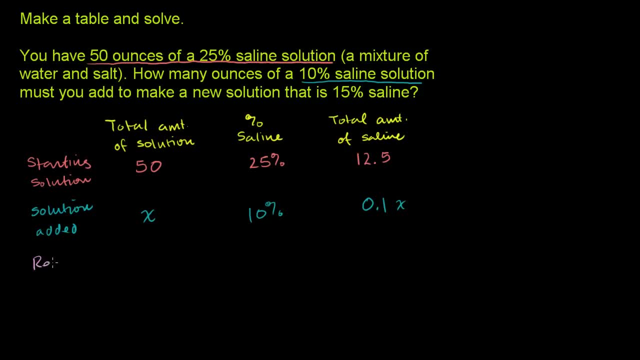 So let me do this in a different color. Resulting solution. Resulting solution: Well, if we started with 50 ounces and we add x ounces, we are going to end up with 50 plus x ounces. That's our total volume of the resulting solution. 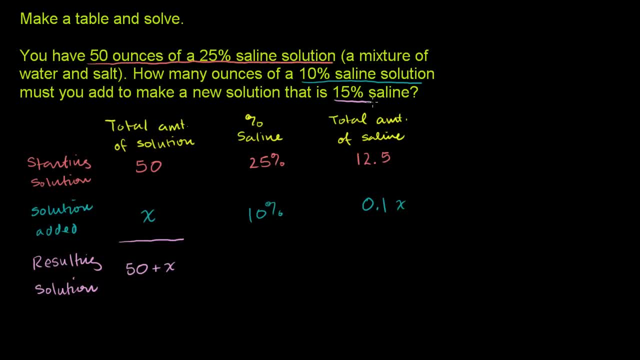 What percent saline is it? Well, our goal is to make a 15% saline solution, So it has to be 15% saline. Now, what's the total amount of saline? And this is kind of the main, I guess box, or the main cell. 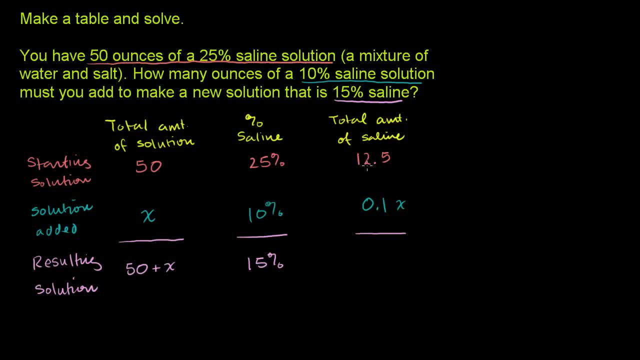 in this table. There's two ways to get to the total amount of saline. in the solution One, we could just multiply the percent saline times the total volume. So we could do that. Let me write that. So it's 0.15 times 50 plus x. 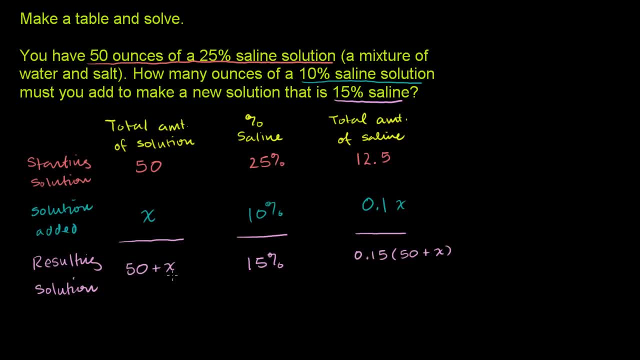 All I did. I multiplied the percent saline times my total volume. That's one way to get the total amount of saline. The other way to get the total amount of saline is to add these two numbers. The 50-ounce solution had 12.5 ounces of saline. 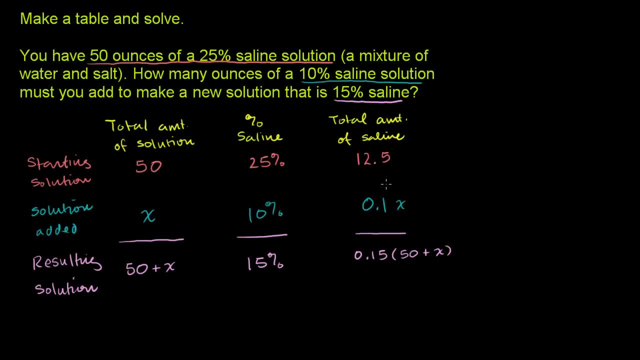 We added 0.1x ounces of saline. So if we add these two numbers, it should also be equal to the total amount of saline. So this has to be equal to the sum of these two things. It has to be equal to 12.5 plus 0.1x. 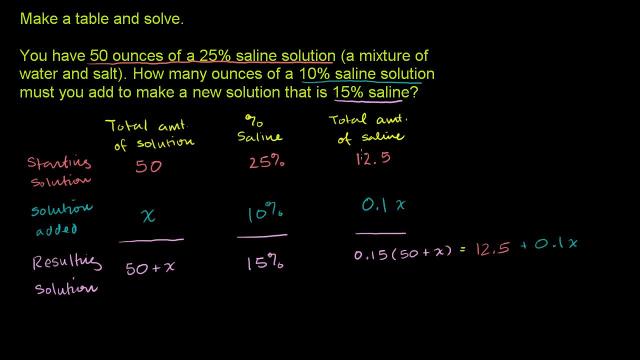 And just like that, because 15% of this has to be the same thing as the sum of this. we have one equation and one unknown, And we can solve for x, which is what we need to solve for. How much solution do we need to add? 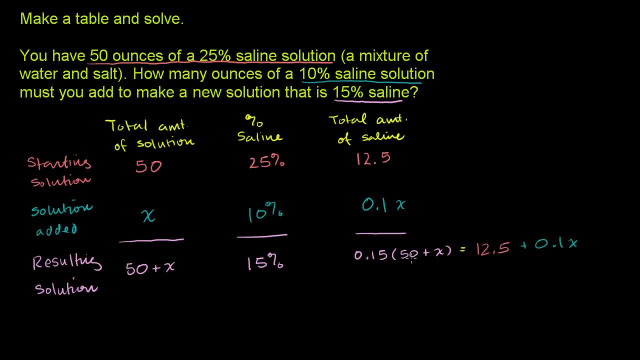 So let's just do that. So 0.15 times 50, let's see if that's 7 and 1 half, if I'm doing that right. Yeah, because 0.15 times 100 would be 15.. 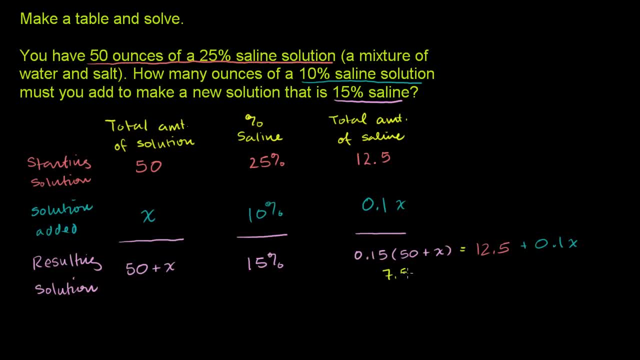 So this is 7.5.. This is 7.5 plus 0.5.. 0.15x, that's the left-hand side, is equal to 12.5 plus 0.1x. Let me scroll to the right a little bit. 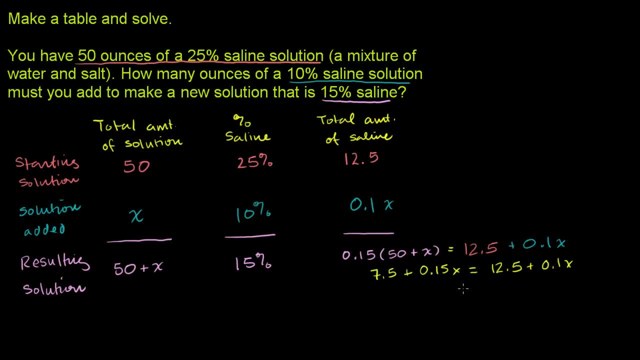 Is equal to 0.1x. Now we can subtract 7.5 from both sides of this equation. I'm doing a new color. So if we subtract 7.5 from both sides of this equation, the left-hand side that cancels out. 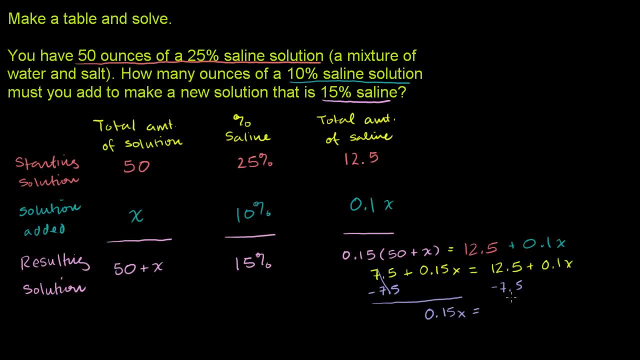 We're just left with. 0.15x is equal to 12.5x, 12.5x, 12.5x, 12.5 minus 7.5 is just 5. 5 plus 0.1x. 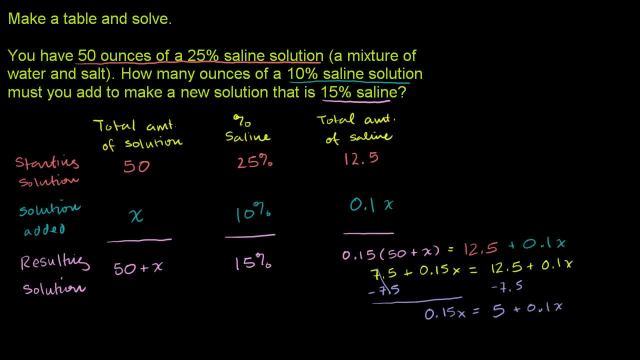 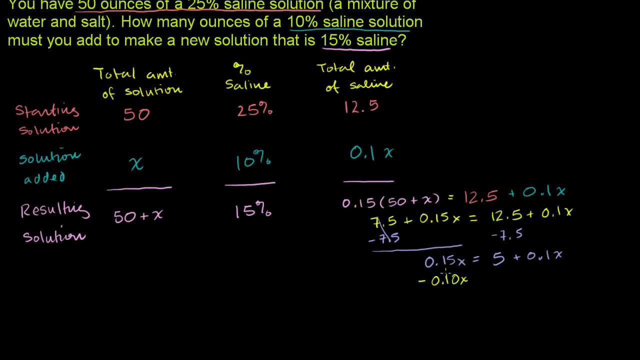 Now we could subtract 0.1x from both sides of this equation. Let me scroll down a little bit. So let me subtract 0.1, or I could say 0.10x from both sides of this equation minus 0.10x. 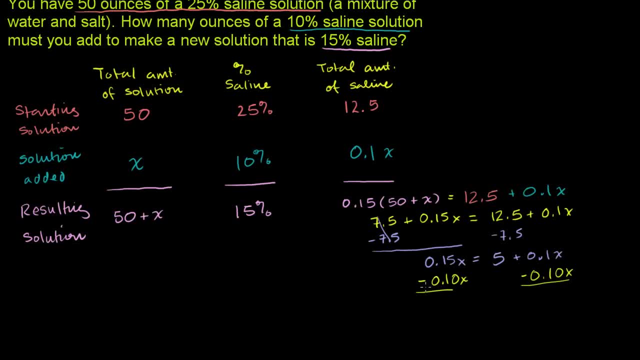 These are the same number, So they cancel out The left-hand side we just end up with. 0.05x is equal to 5. And now we just divide both sides by 0.05.. So divide both sides by 0.05.. 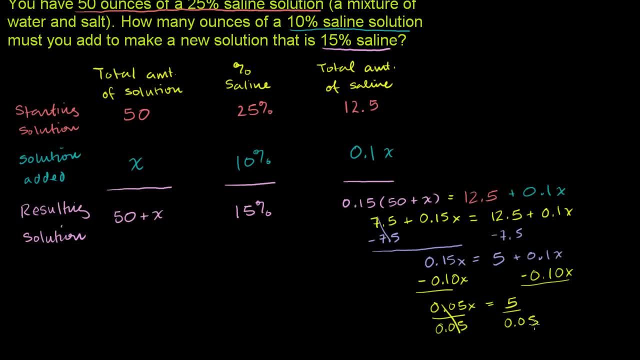 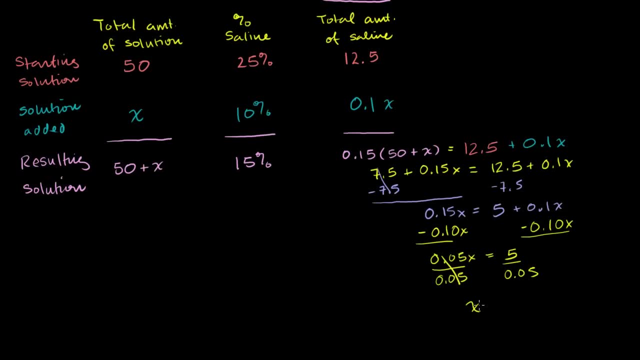 And we get: x is equal to 5 divided by 0.05.. That's the same thing as 5 divided by 1. 20th, or the same thing as 5 times 20.. So we get: x is equal to 100.